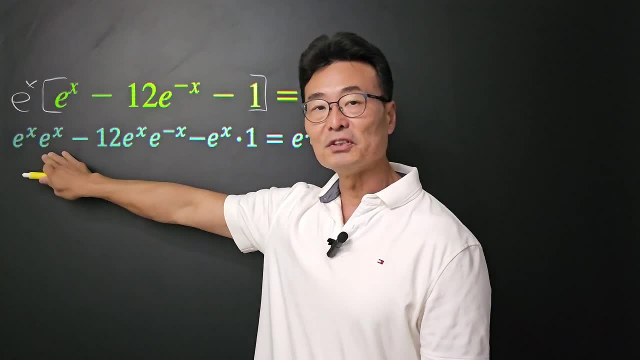 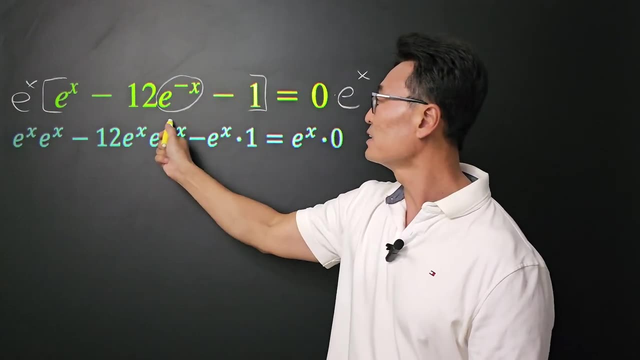 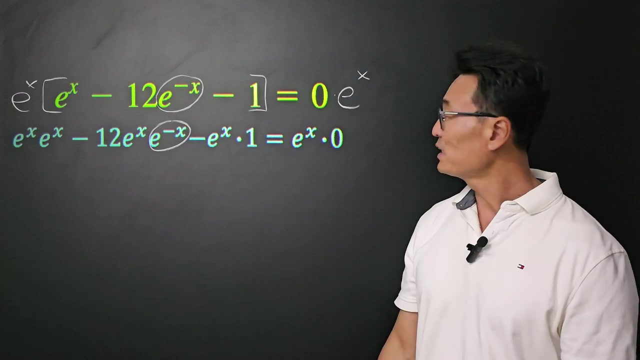 multiply into the parentheses we get e to the x times e to the x minus 12 times e to the x times e to the negative x. And notice that e to the negative x is that e to the negative x minus e to the x times 1 is equal to e to the x times 0.. Next, if we combine e to the x times e to the x, 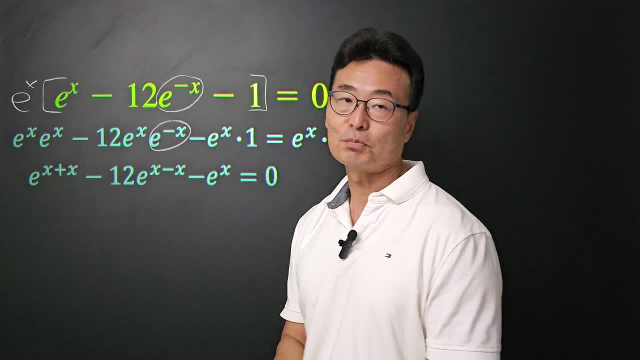 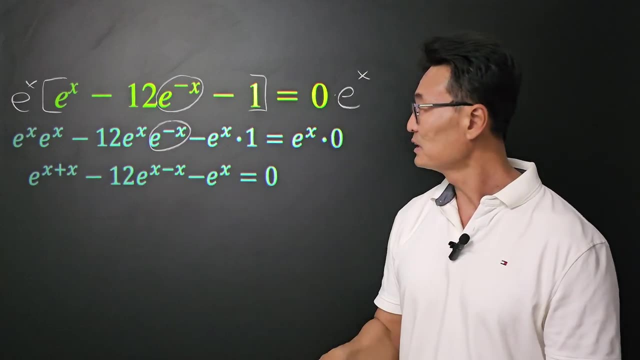 that same thing as e to the x plus x. we're just adding the exponents, And then, of course, we have the x minus x. So we have e to the x minus x. Again, we add the exponents, And then 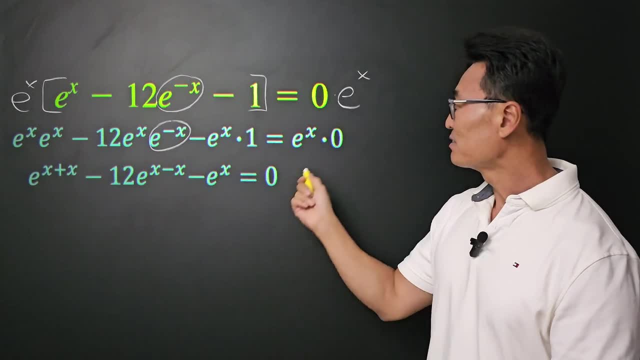 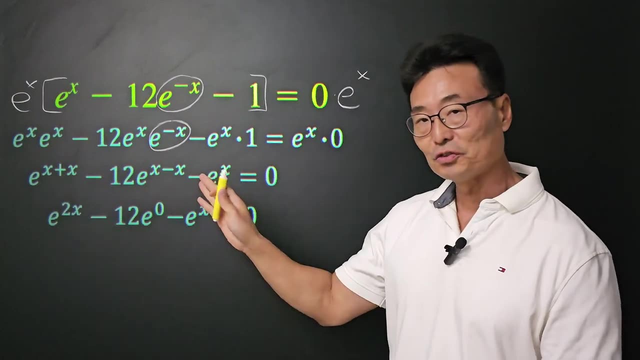 e to the x times 1 is Of course e to the x, And on the right side it's just going to be 0. Then x plus x is 2 to the x or 2x, And then x minus x is 0 power, And we still have that e to the x. 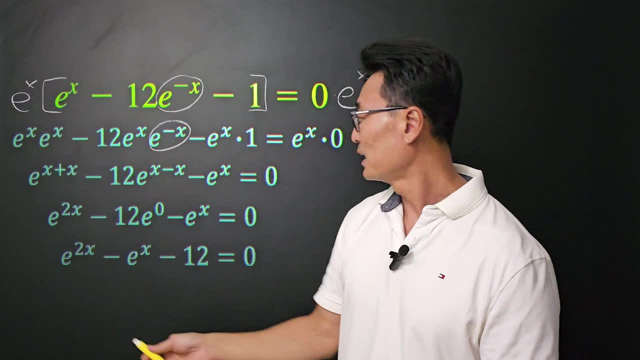 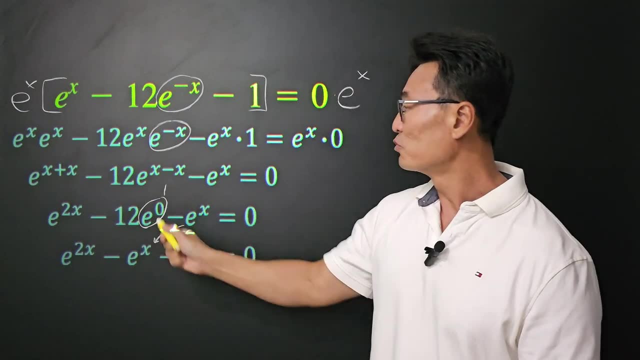 Next we have e to the 2x in the front And what I decided to do was put that negative e to the x here in the middle position, And e to the 0 is 1.. So I decided to put the 12. 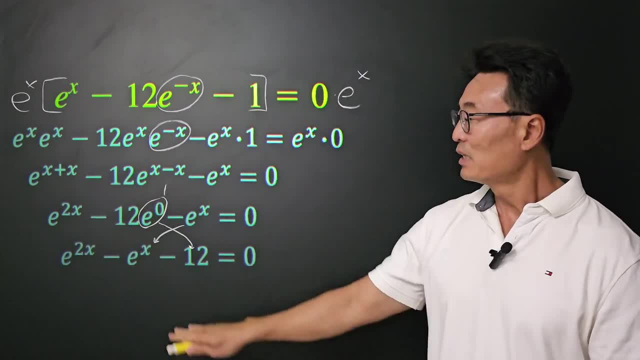 in the third position And then e to the 0 is 1.. So I decided to put the 12 in the third position. Next we're going to be factoring this, And to factor this I'm going to be using a little. 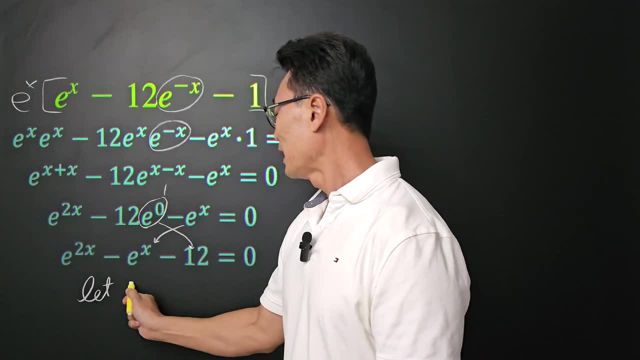 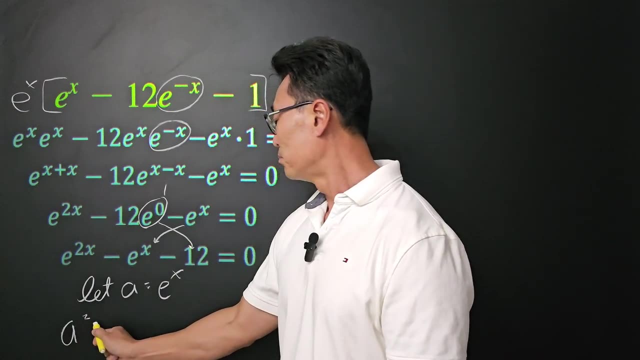 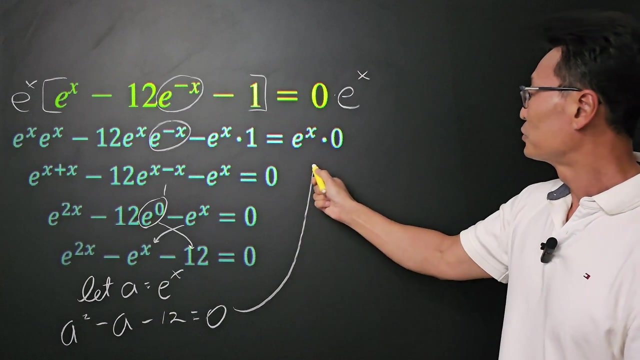 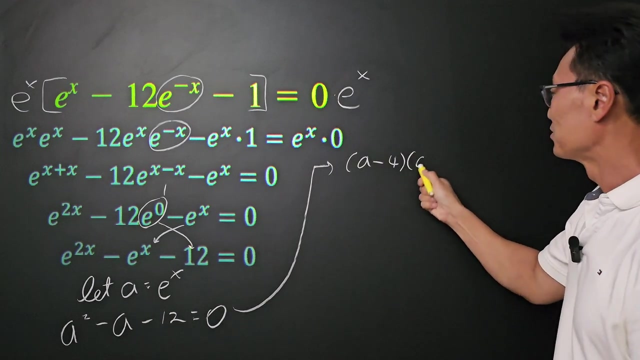 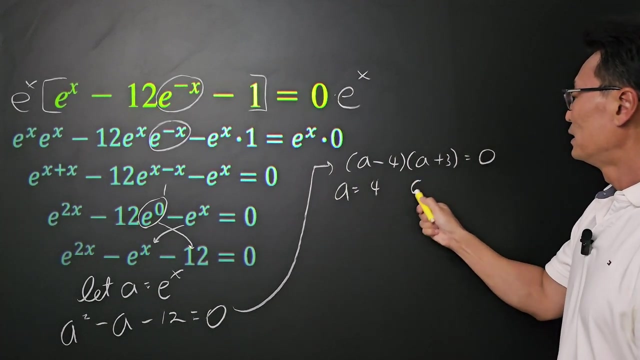 substitution. So let's let: a is equal to e to the x, Then we now have a squared minus a. minus 12 equals to 0. And if we were to go ahead and factor this equation here, then we get minus 4 times a. plus 3 equals to 0, where a equals to 4 or a equals to negative 3.. 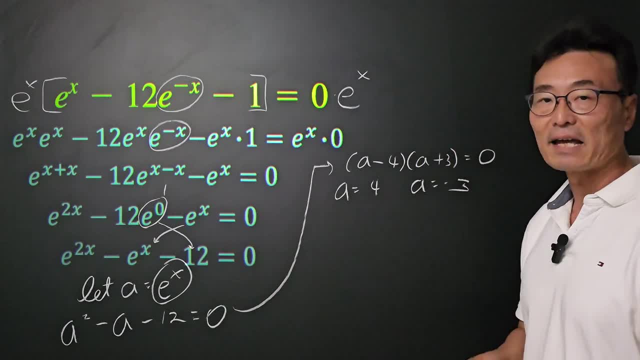 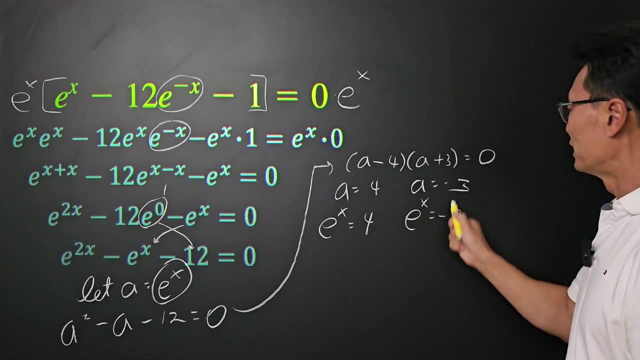 Now it's time to go back and plug in the e to the x for the a value that we have. So we have: e to the x equals 4 and e to the x equals negative 3.. Remember, whenever you have an exponential function, e to the anything, power can never be a negative value. 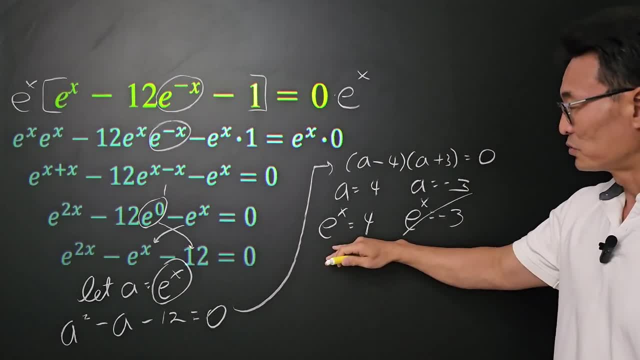 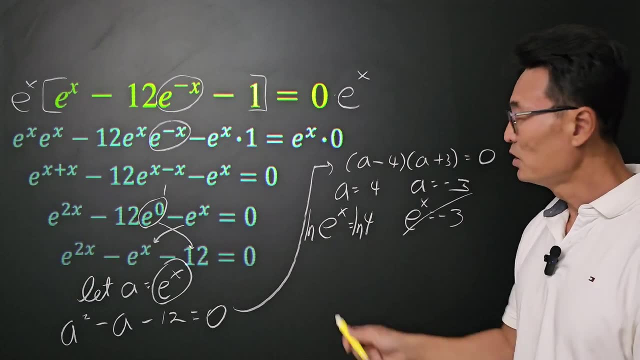 So this one we're going to ignore. We're going to focus on this: To find the x value. what we could do is we could take the natural log of left and the right side, where the natural log and the e will cancel out, And we're left with only x on the left side.